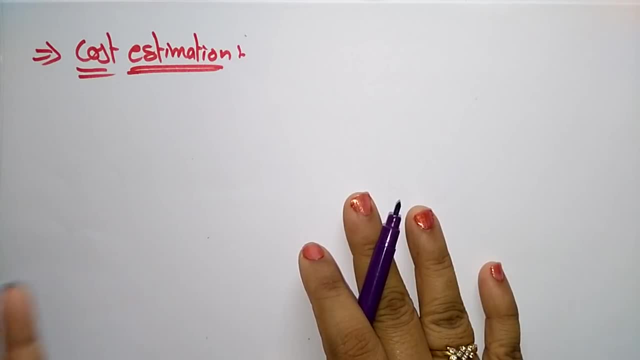 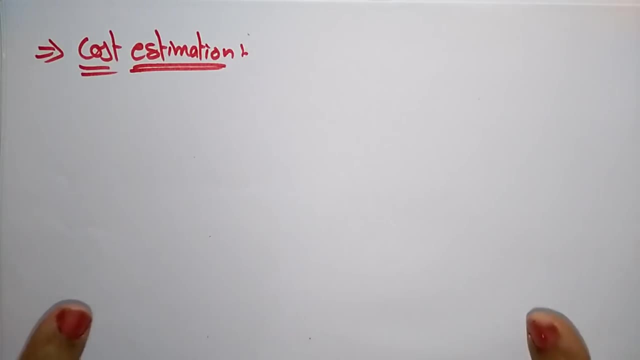 project, because if you didn't have a clear idea about the cost of that is going to be made on your project, that you have to be know because you have to charge from the customers, you have to give some code to the customers to before developing a project. so that has to be. 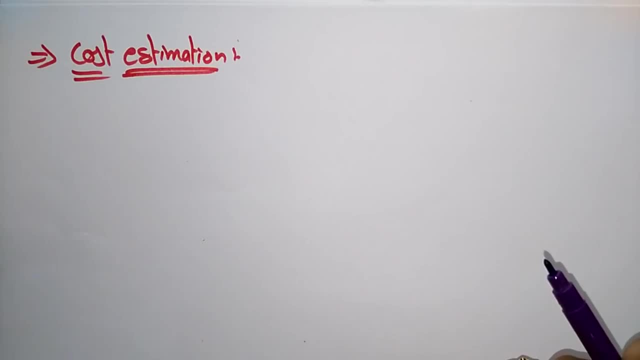 estimated at the starting point of your project only. so whenever the customer is wants to uh, given a project to a developer to develop a project first, he has to give some estimation. that is a software project. planning should be there. so the planning is the size of the estimation cost. 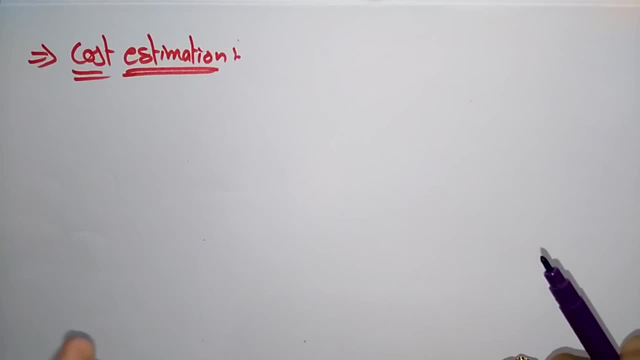 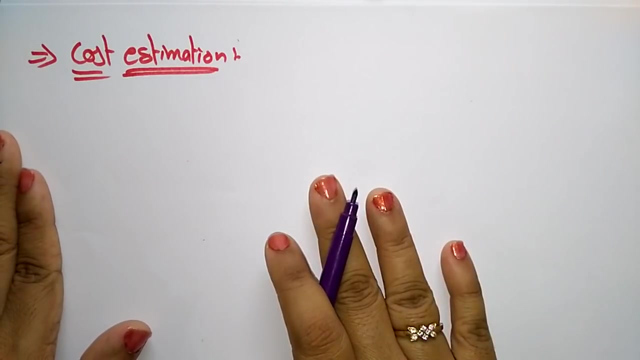 estimation, resource requirements, everything they have to be planned before starting of the project only. so now let us see the cost estimation, how it is going to be: uh, calculate of a. uh, calculate the cost of a project. so there are number of estimation techniques have been developed, okay, so so many number of 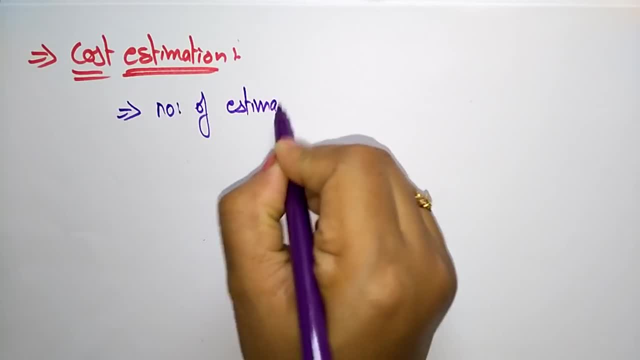 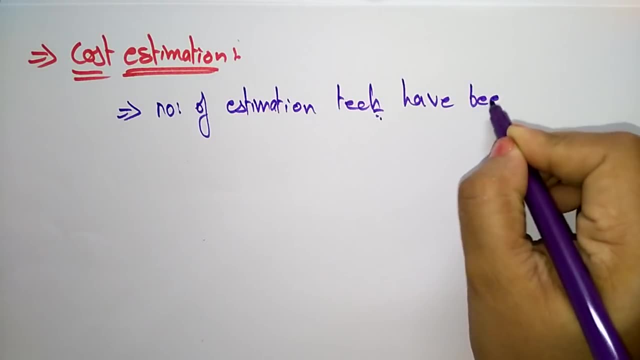 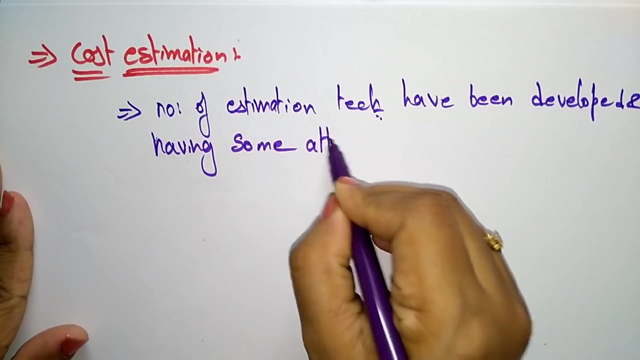 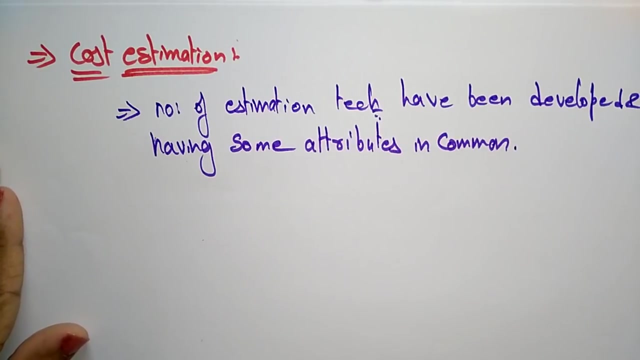 number of estimation, that is, a cost estimation techniques. cost estimation techniques have been developed and ha and having some uh attributes in common have been developed and having some attributes in common. so whatever the technique you have taken to develop a project means whatever the technique that you are using for cost estimation to develop a product, uh, every technique have some common. 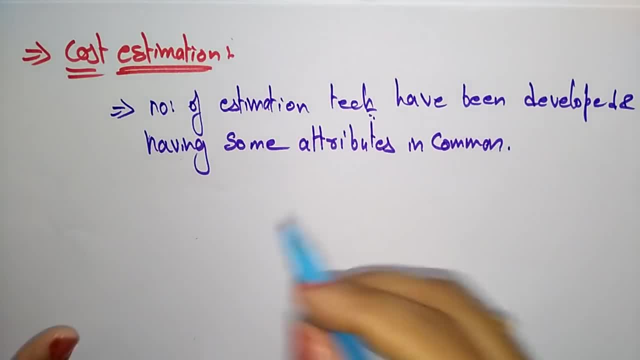 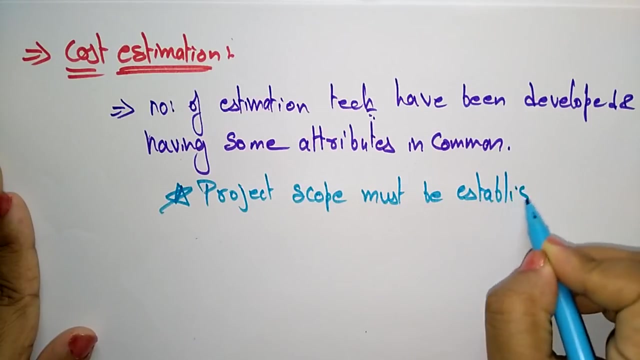 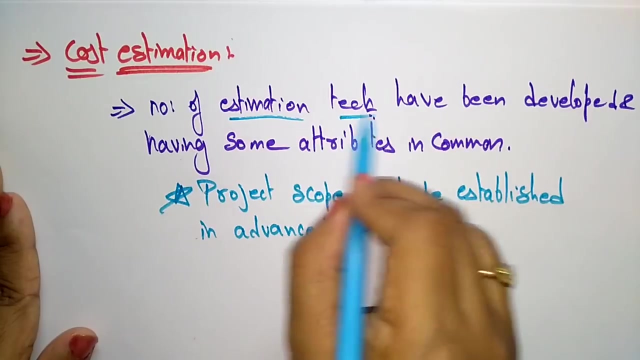 attributes. whatever the technique you have taken that has to follow these common attributes. that is, that each technique has to think about the project scope. that must be established in advanced, in advanced. so whatever the cost estimation technique you have taken, so that cost estimation technique have attribute like it has to think about the project scope must. 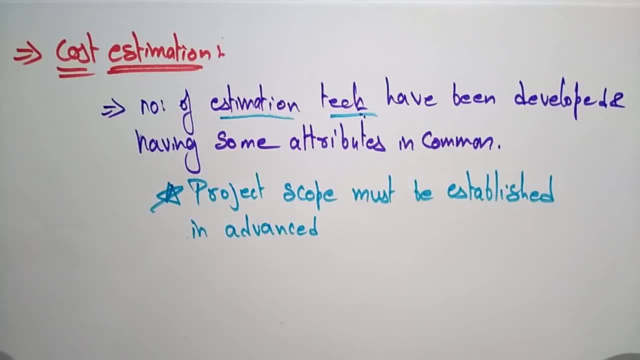 be established in advance. so starting itself. only you have to be declared what is the project scope means within this limited time: one year, two years, three years or five year means it's a six months, two months, three months, like that. the project scope must you have to be established in. 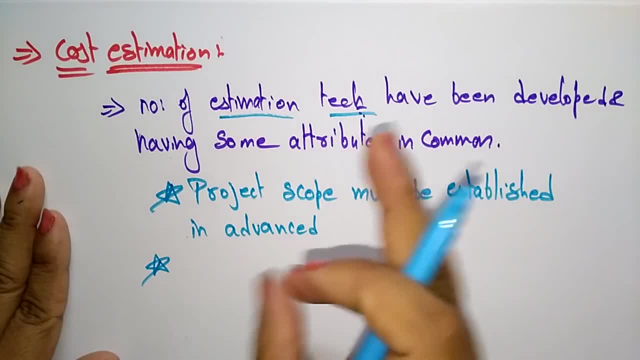 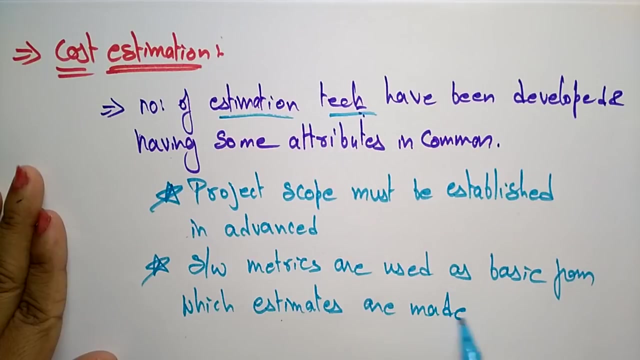 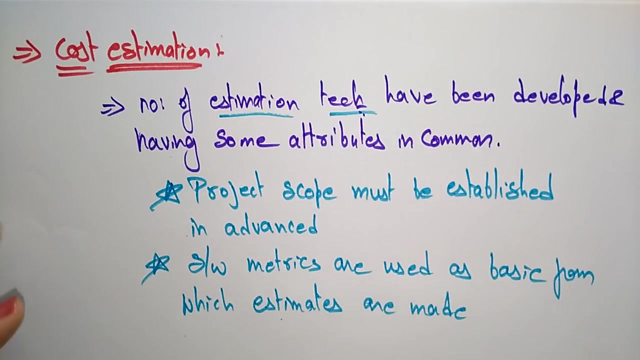 in advance. so, whatever the technique you have taken, this point has to be followed. in the same way. software metrics are used as basic from which estimate or made, which estimates or made. so the software metrics are used as basic from the estimates or made. whatever the estimation, cost estimation you have taken, you have to see the software measurements. so, whatever the 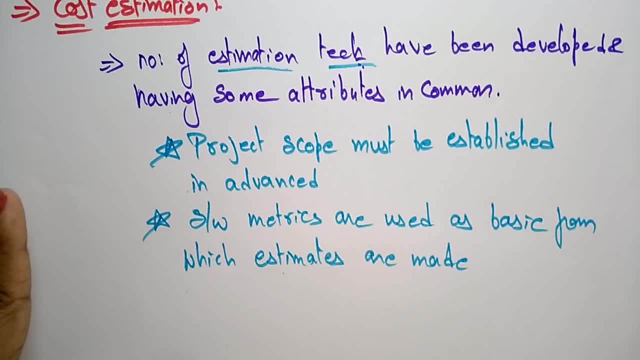 softwares you are using, what is the cost that it measures the cost of that software. you are using the tools that you are using so that you have to be known. so for every cost estimation technique and the project is divided into. project is divided into small pieces. 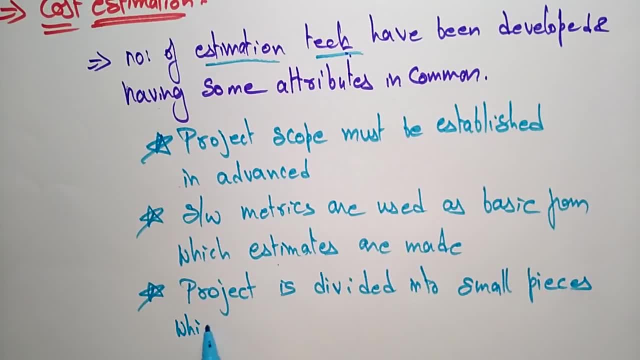 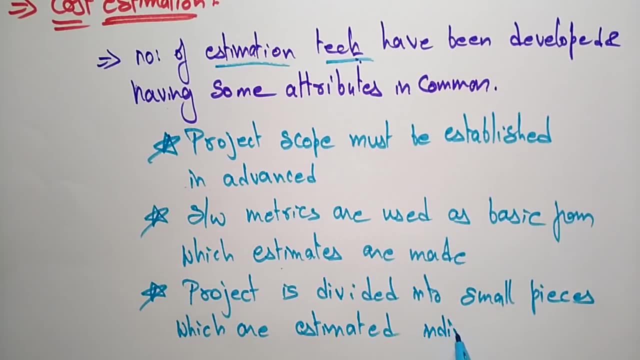 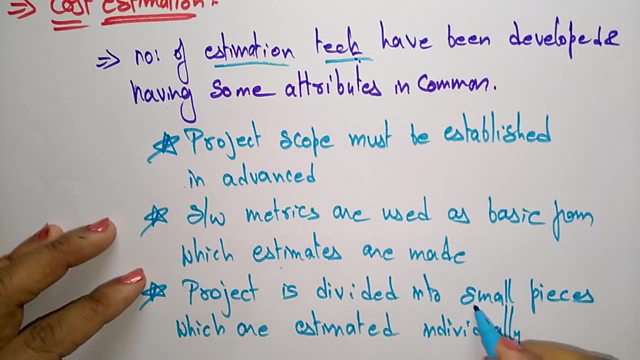 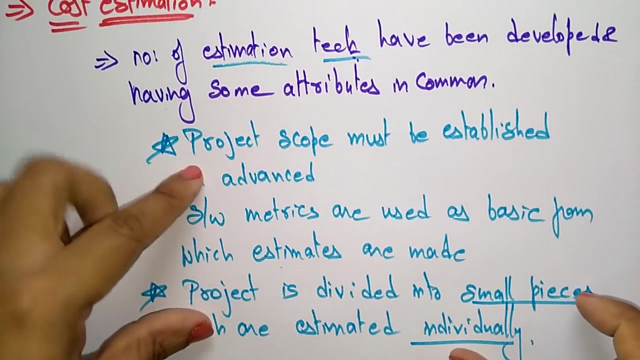 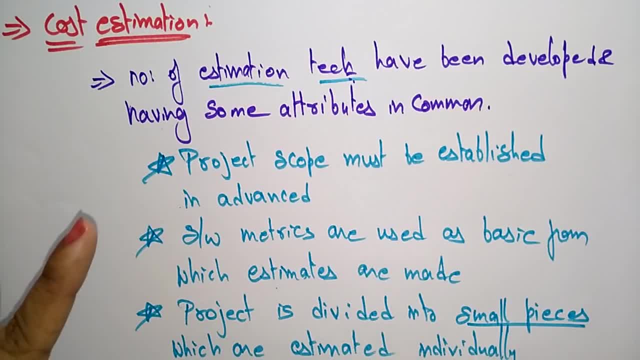 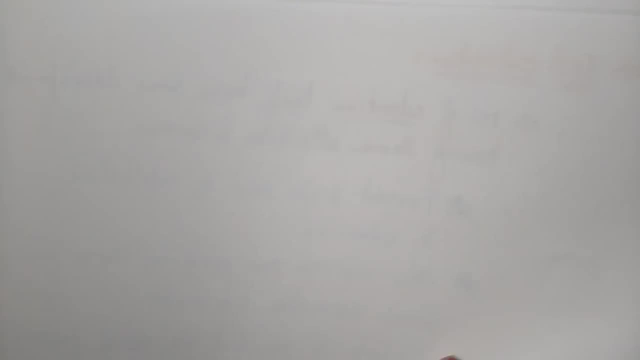